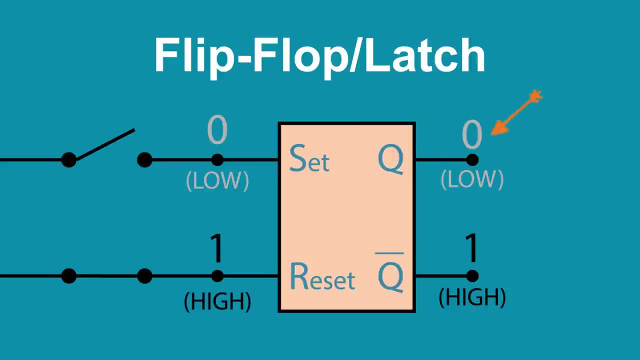 high, the output will change to low. Other changes of the inputs do not affect the output. Reset can go high and low and won't do anything as long as the output is low. After set goes high. once changing the output to high, set can go high or 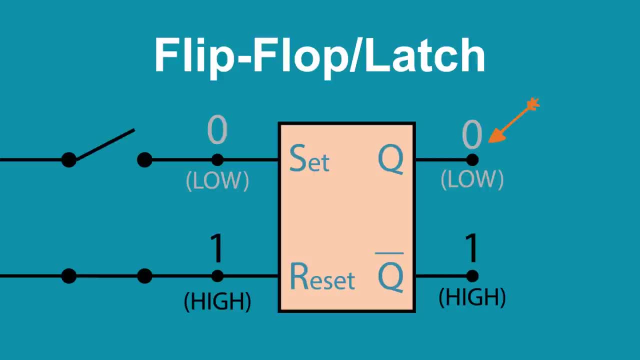 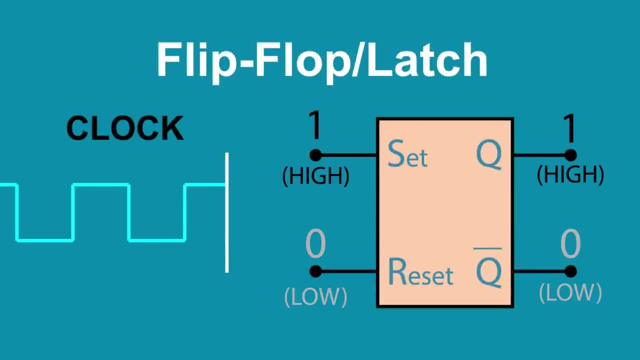 low without changing the output until the output is reset low again. This change frequently requires a clock pulse, meaning there is an external clock signal that ticks and tocks and the inputs only change the output when the clock ticks. Now there's some contention about what differentiates a flip-flop from a latch. 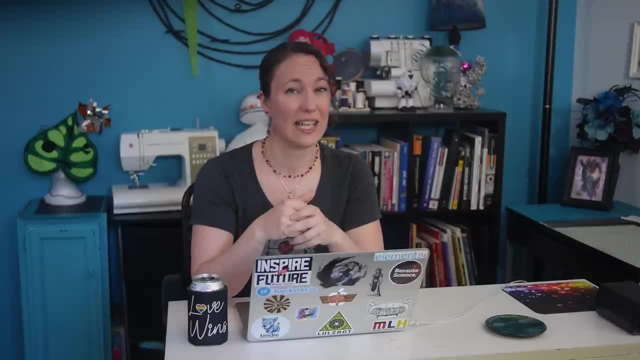 Some say it depends on the presence of a clock signal. I have yet to find a definitive answer and often see the terms used interchangeably. If you feel passionate about it, feel free to discuss it in the comments. In the meantime, back to shift registers. 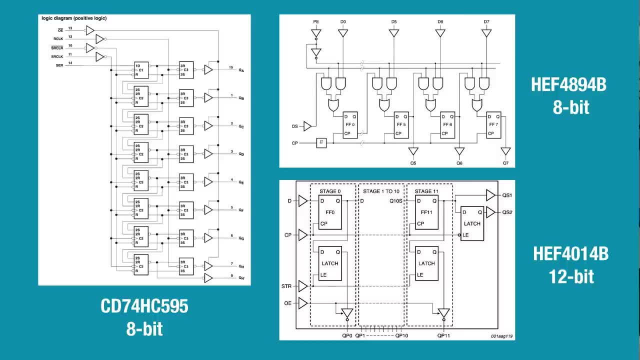 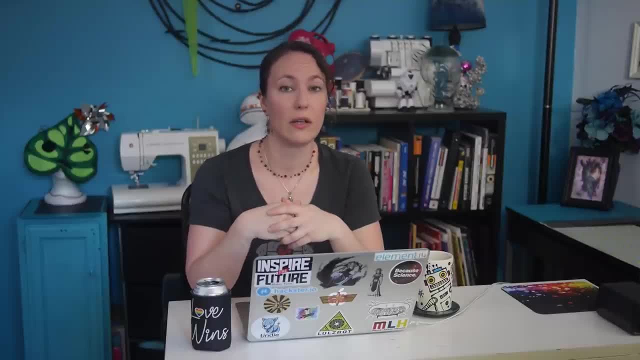 In a shift register. the flip-flops and latches make up stages. Each can hold one bit of data. A bit is either a 1 or a 0,, 1 being a high voltage signal and 0 being a low voltage signal. 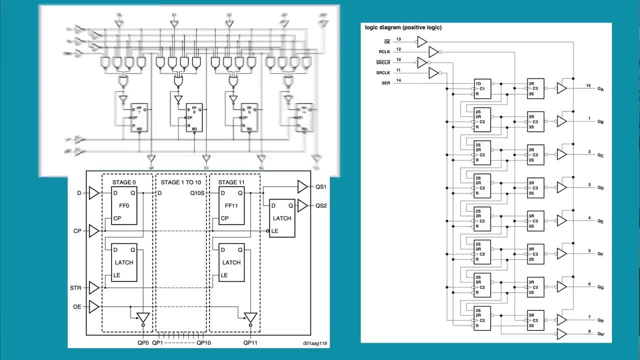 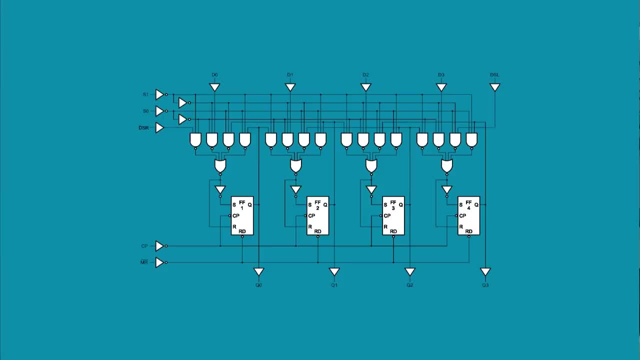 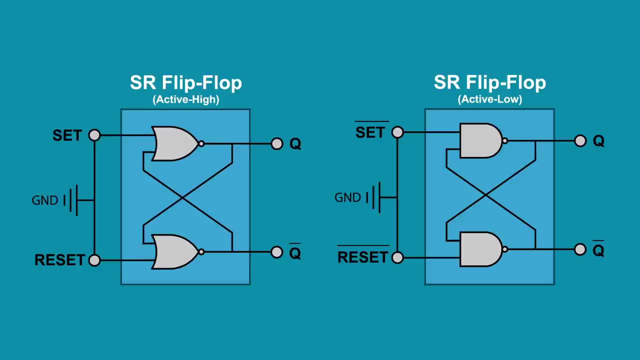 The number of bits a shift register can process, be it 4-bit, 8-bit or 12-bit, corresponds with the number of latches or stages it has: 4,, 8,, 12.. In my flip-flop video we saw that they have memory because the output of one logic gate is 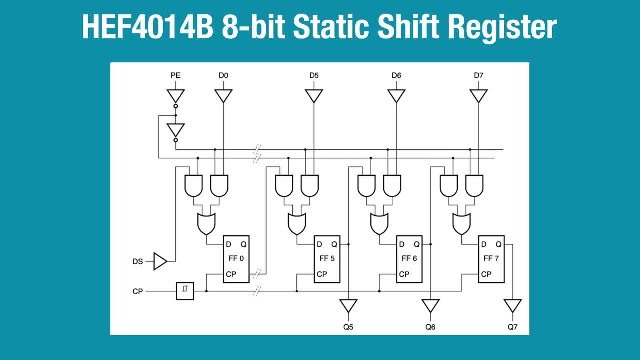 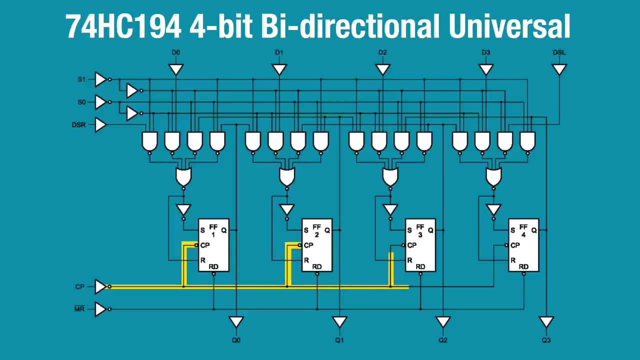 connected back to the input of the other logic gate. Similarly, a shift register has memory because the output of each latch is connected to the input of the next latch. Each internal flip-flop is also connected to the external clock pin. The flip-flop's inputs will only change its outputs on the next clock pulse. 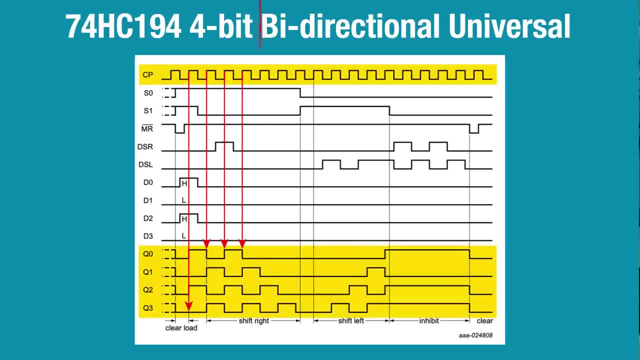 You can see on this timing diagram, the state of any output only changes on the edge of a clock pulse. Here, even if the signals from inputs D0-3 change, outputs Q0-3 won't change until the next rising edge of the clock pulse. So looking back at this logic diagram, 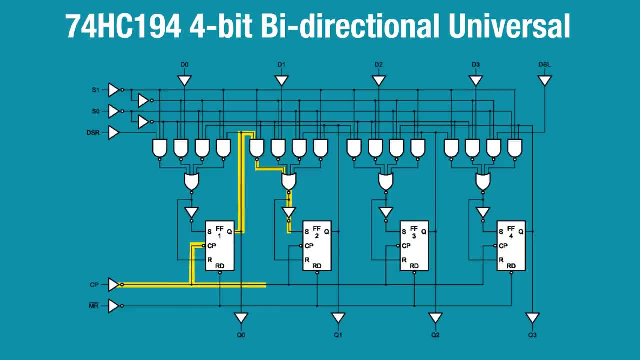 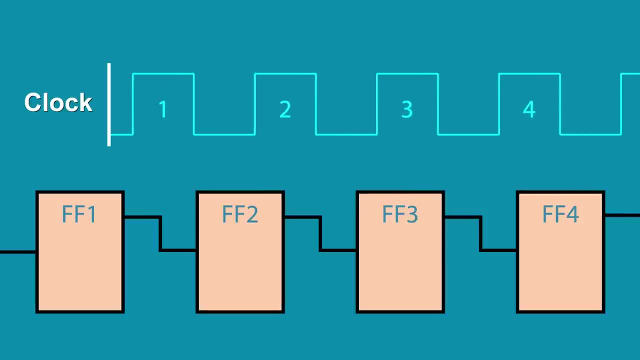 the output of a flip-flop will only affect the next flip-flop when the clock signal pulses. This is where the shift in shift registers comes from. A bit of data will be latched in the first and will shift to the next flip-flop on each consecutive clock pulse. So in a 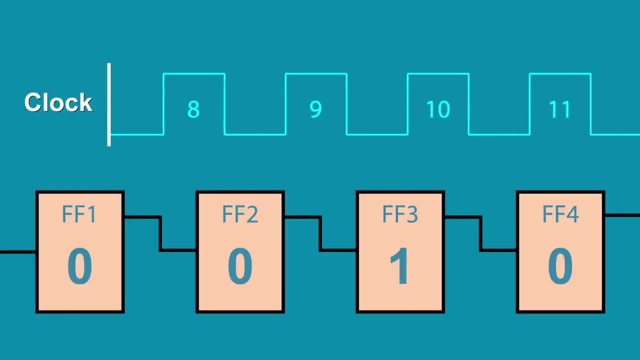 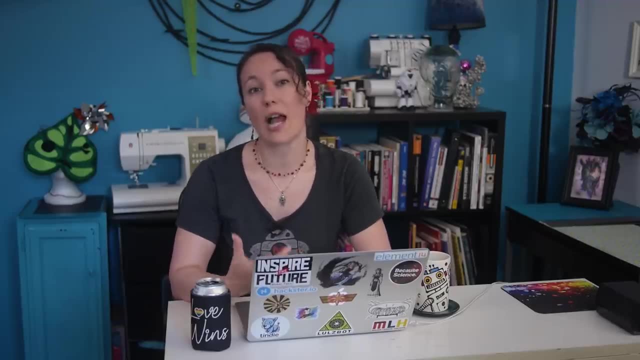 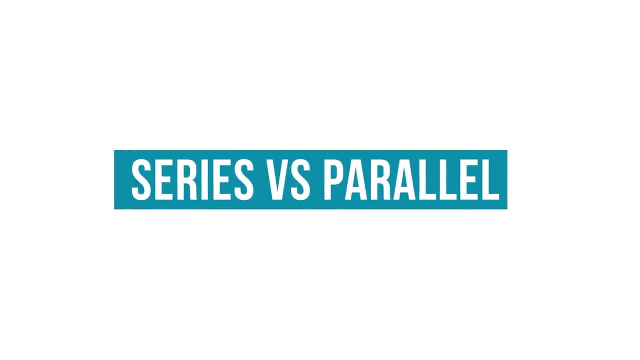 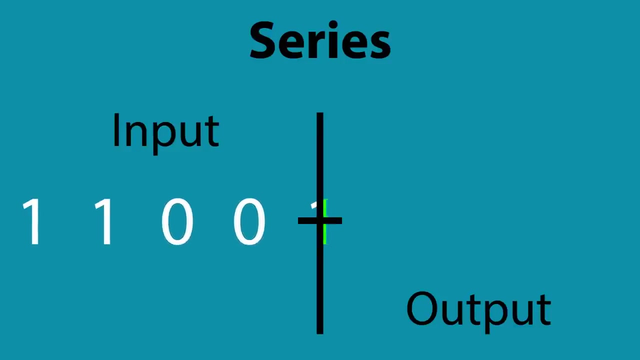 four-bit shift register. it takes four clock pulses for a bit of data to move across all positions In a shift register. data can be input or output in two different ways: in parallel or in series. In series, the ones and zeros or high and low signals are processed one at a time. 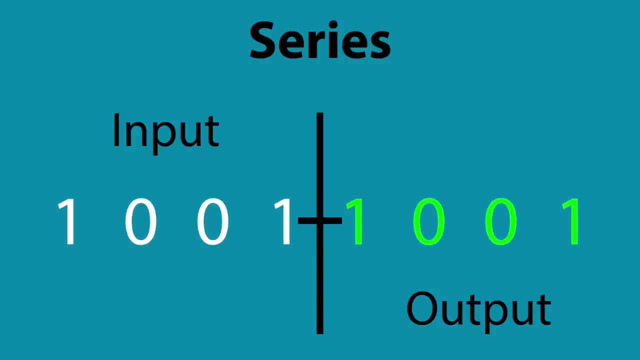 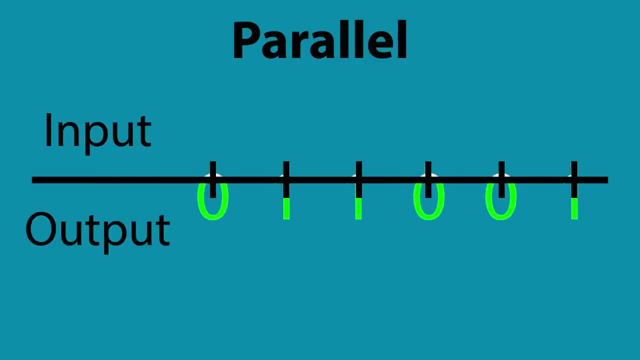 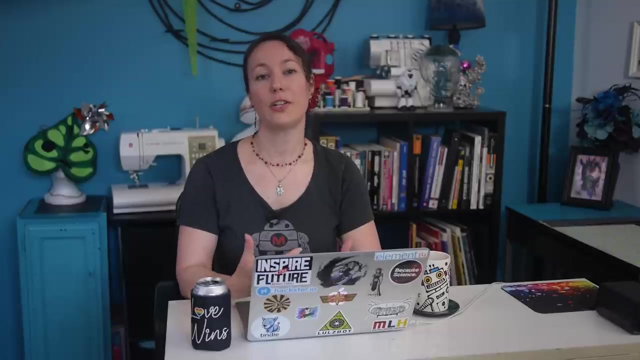 in order, requiring only one input or output. In parallel, a set number of bits of data can be processed all at once, but this requires multiple inputs or outputs- one per bit of data. Shift registers have four possible modes of operation, While 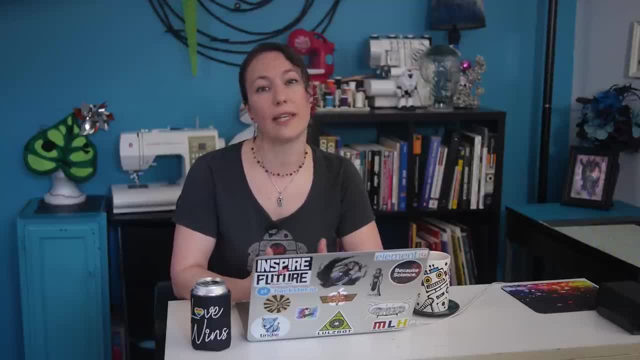 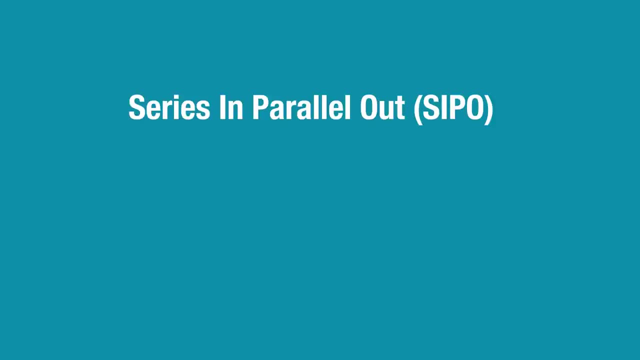 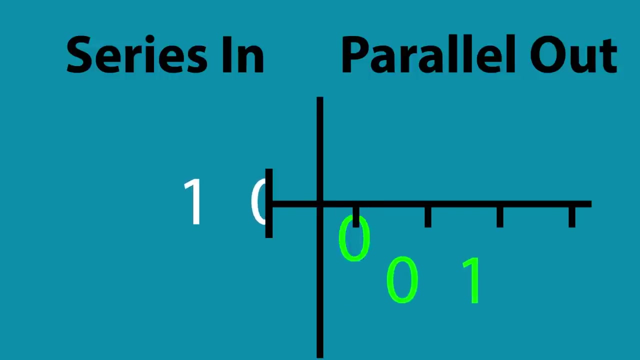 most chips are capable of at least two modes. they're not typically capable of all four. The four modes are: series in parallel out, series in series out, parallel in series out and parallel in parallel out. For series in parallel out mode, data comes in one input and 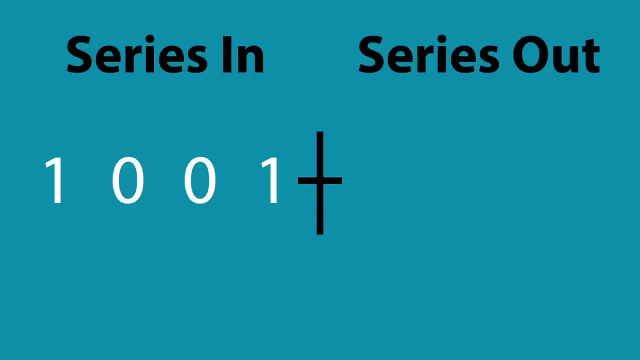 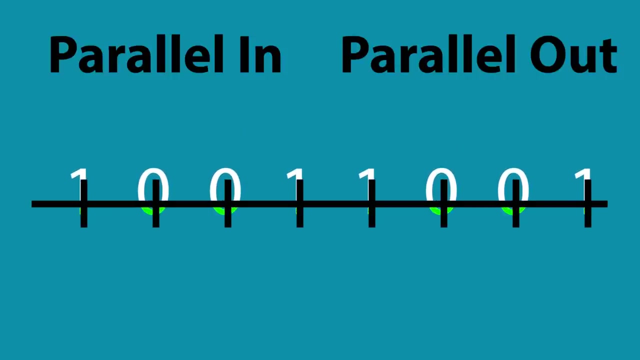 shifts across multiple outputs. Series in series out: has the same data coming in from one input going to one output. Parallel in series out: has data coming in multiple inputs which shifts to be sent out one output. Parallel in parallel out. has data coming in multiple inputs going out to: 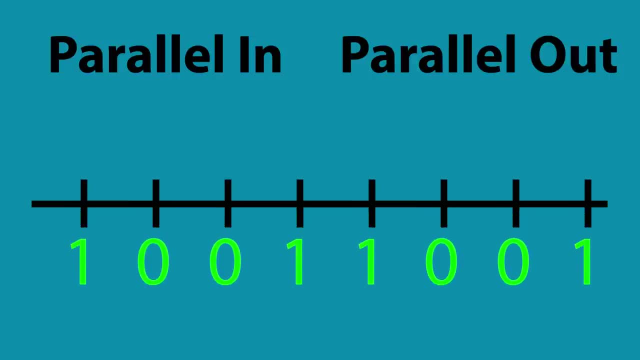 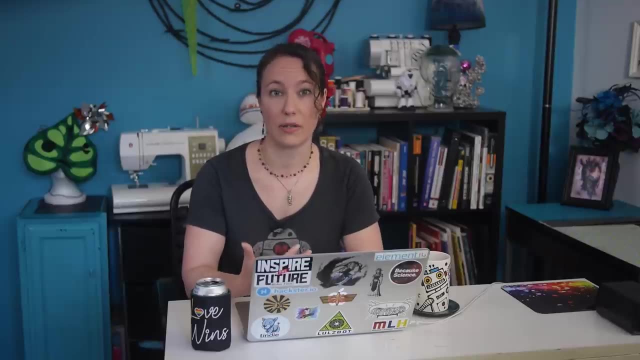 typically the same number of outputs. What's interesting about shift registers is the clock signal. It's seen in other ICs that the clock is a constant pulse, an oscillating signal that goes high and low at a steady rate, like a metronome. 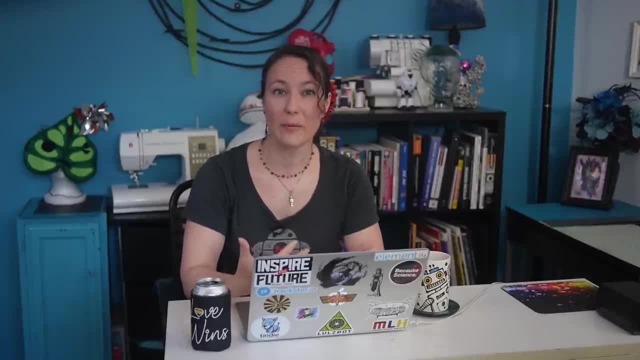 In shift registers that's not always the case. The clock pin can be used more like an enable pin or momentary switch, causing data to selectively be shifted from the inputs or to the outputs. However, shift registers also often have other enable pins. 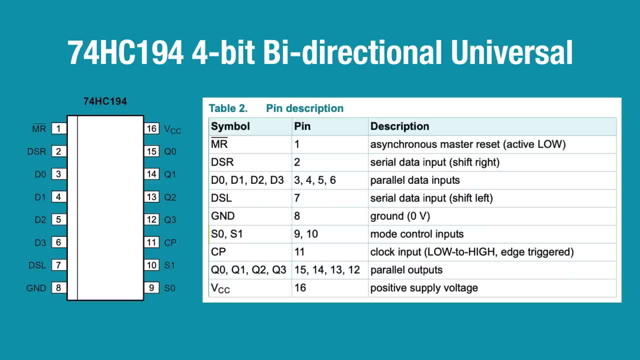 I'll show you an example. This universal shift register can operate in serial-in-parallel-out mode using one serial input, either DSR or DSL, or it can operate in parallel-in-parallel-out mode using the four parallel inputs D0 through 3.. 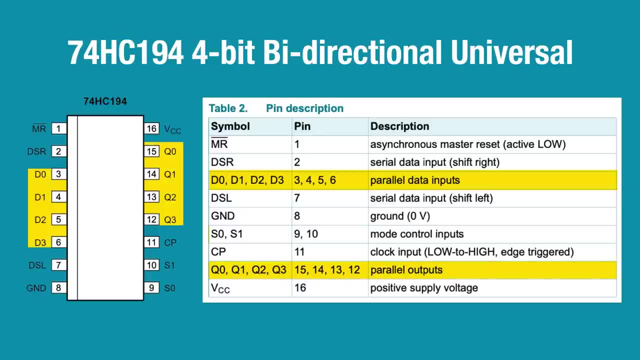 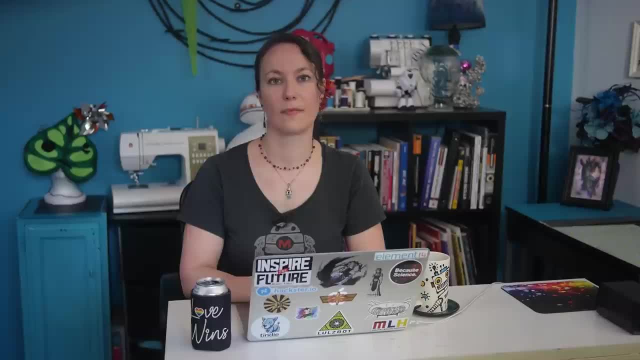 In either mode the four parallel outputs Q0 through 3 are used. Pins S0 and S1 act like enable pins In most shift registers. this is the case In most shift registers. bits shift left to right but universal shift registers have. 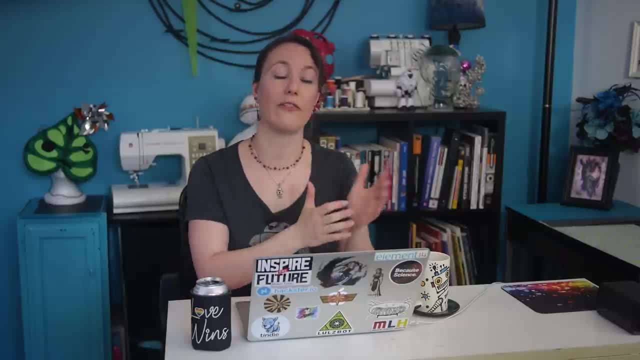 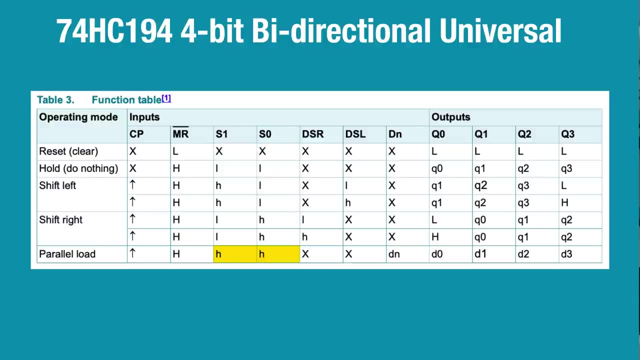 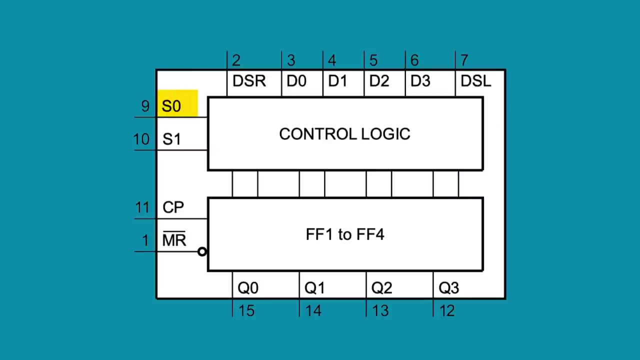 an additional serial input where bits shift right to left. S0 and S1 each enable one of the serial inputs or together can enable the parallel inputs In serial mode. when S0 is high, serial input DSR- is enabled. 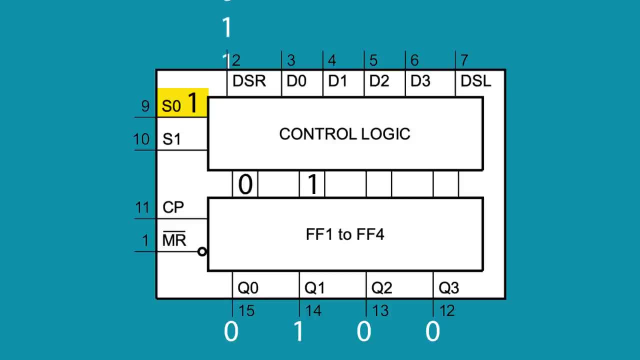 Any data at that input shifts left to right. When S1 is high, serial input DSL is enabled. Any data coming in DSL is shifted right to left through the registers to the outputs. When both S0 and S1 are high, the chip is put in parallel mode. 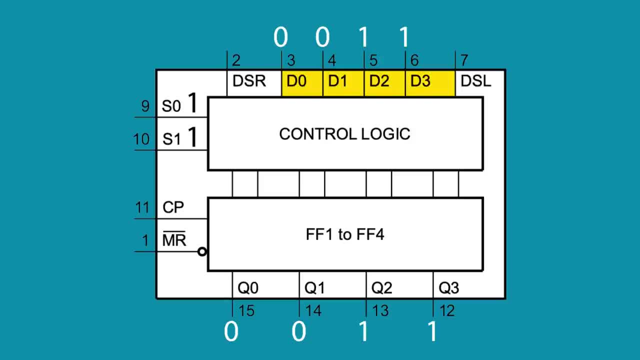 Data at D0,, 1,, 2, and 3 is shifted to chorus mode. When S0 and S1 are high, the chip is put in parallel mode. They are then moved to the corresponding outputs Q0,, 1,, 2, and 3.. 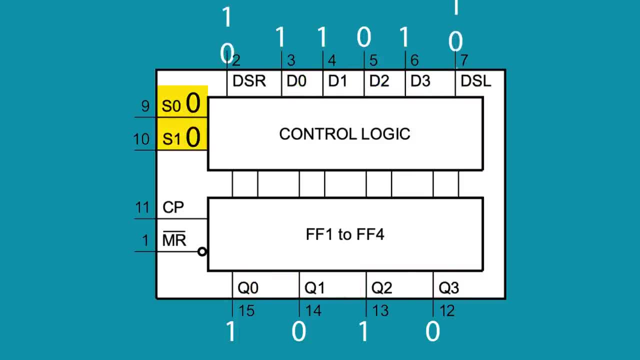 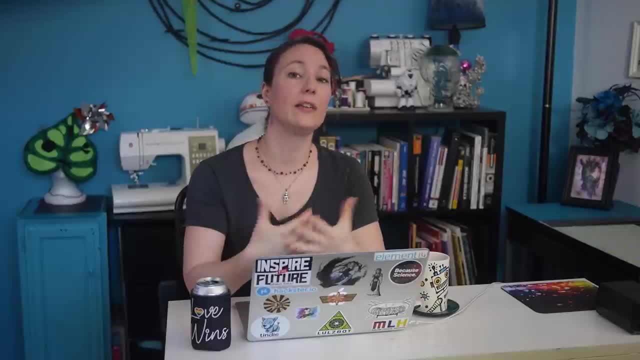 Both S0 and S1. going low effectively disables all the inputs. So the outputs will not change, no matter the input data. When any of the inputs are enabled, a clock pulse is still needed to transfer a bit from an input into the shift register. 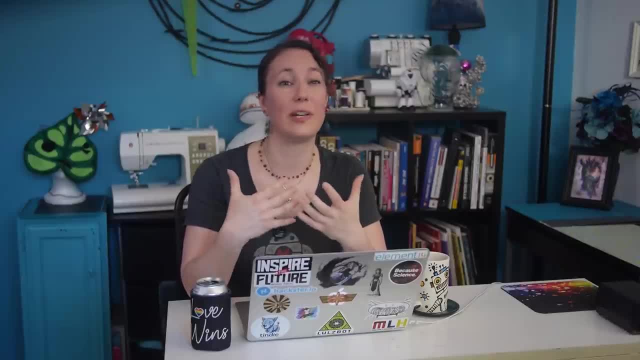 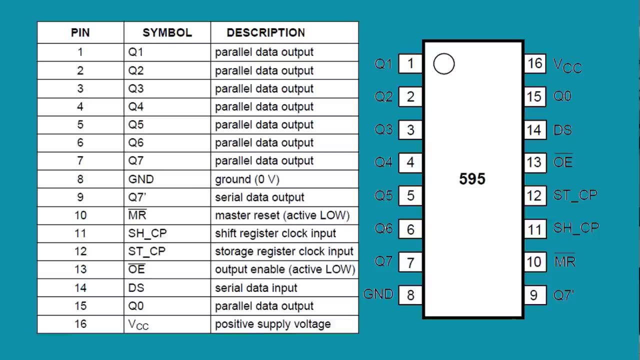 To make things even more confusing and complicated, some shift registers appear to have two clock pins. in this 8-bit serial in parallel out shift register there are two clock pins, one labeled shift register and one labeled storage register, and then the chip also has an output enable pin. the shift register clock pin acts as the